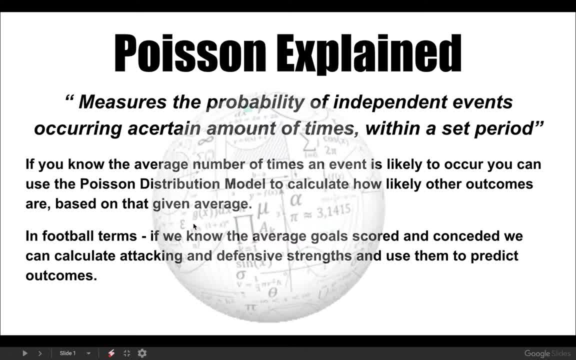 The Poisson distribution model. It's been about a couple of years since my last video, which is a bit unusual for most YouTubers, but I don't class myself as a YouTuber. I have been still betting and doing statistical modeling in the last two years, but life has got in the way of social media and uploading videos, unfortunately. 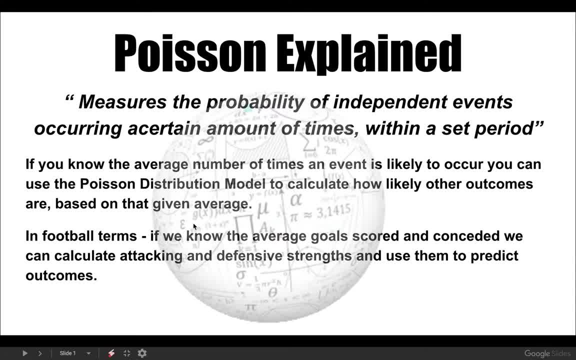 But I came back and checked in on the account a couple of weeks ago and saw the amount of likes and the amount of love that I'd got on the video. so I thought you know what I'll do. another one, because I'm actually back in the swing of things, so I might as well start recording again. 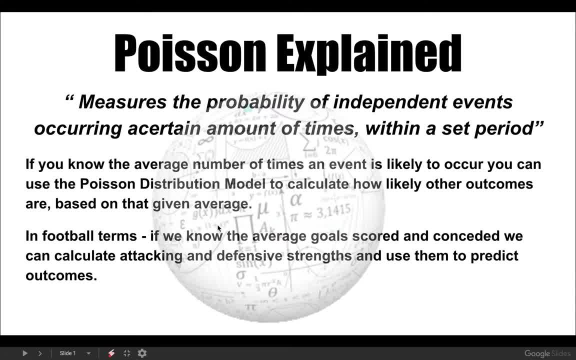 So to briefly talk about what we are looking at, the Poisson distribution model. you can Google it. There are tons of great episodes on YouTube. There are tons of great tutorials about what the Poisson distribution model is, But in a nutshell, it measures. 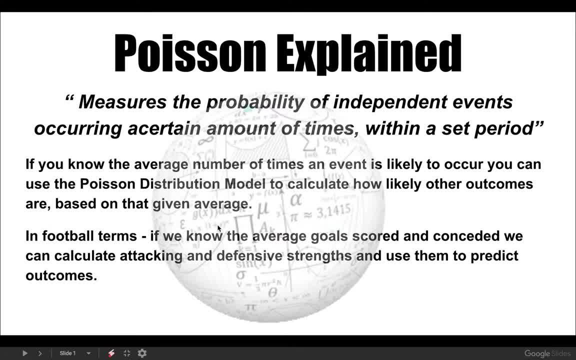 It measures the probability of an independent event occurring a certain amount of times- apologies for the spelling error- within a set period. So if you know the average number of times an event is likely to occur, you can then use the model to predict how likely other outcomes are based on that given average. 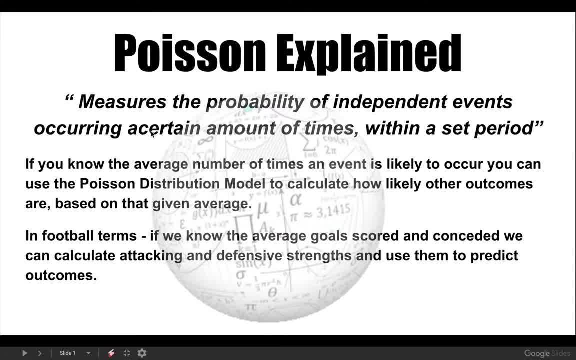 It all sounds like a lot of waffle for anybody who's not that into mathematical modeling. In football terms, if we know the average goals scored and conceded, we can then use them to calculate defensive and attacking strengths of teams and then multiply Those together to come out with some sort of match outcome or some sort of expected number of goals in a given game. 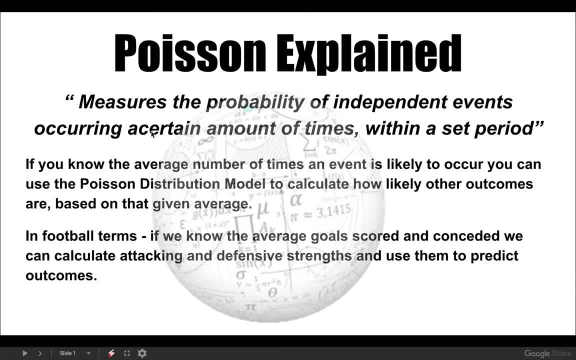 I find it extremely interesting and it's aided me quite a lot in my betting, so I thought we could have a quick look at it and I could talk about a bit of an updated view on it from my last video. Okay, so, firstly, what we need to do is look at 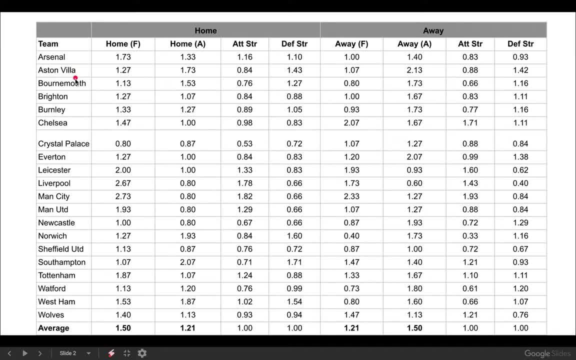 Well, I'll tell you what data set I'm using. first, This is the current English Premier League season and I'm making this video for anyone who's watching in the future, In June 2020, so just after the resumption of play after the coronavirus, which is worth considering when betting at the moment if people are watching it currently. 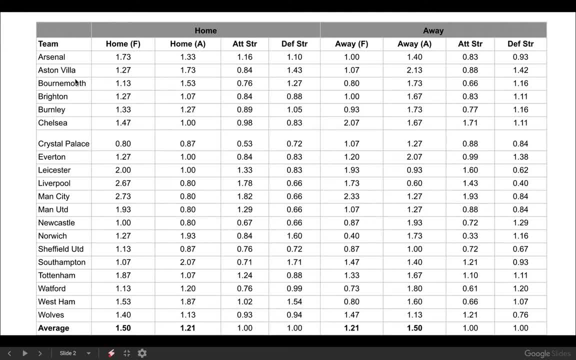 Home and away statistics are not going to carry quite the same weight as they did beforehand. when playing in front of empty stadiums There's still going to be a bit of a bias because of the unusual surroundings, the playing surface, the traveling etc. 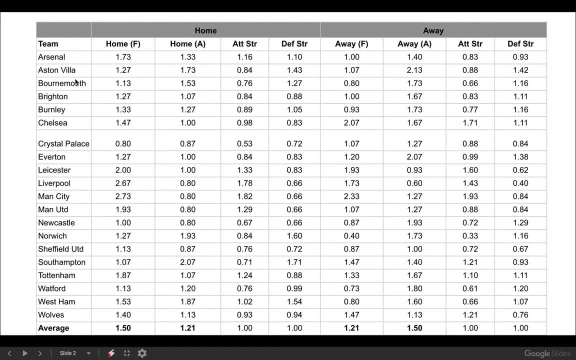 But not quite as much of an advantage- playing at home, I would suggest, as playing in front of a, So that might be worth just considering. But all things equal, let's ignore that and let's just look at the statistics. So we're using data from 1920 in the Premier League. 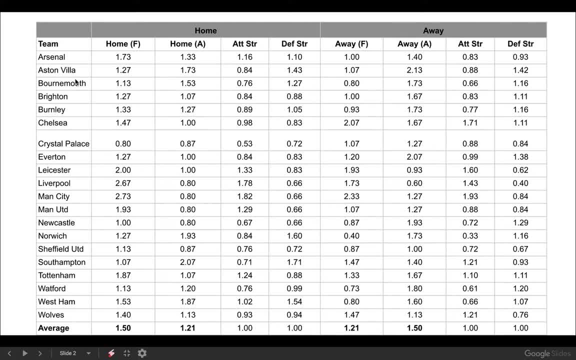 In my previous video I used the previous season's data. That was because I recorded it in the October, I think, and there wasn't, in my opinion, enough data to model. But we're near the end of the season now, so I've used the data from the current season and I've used all of the teams. 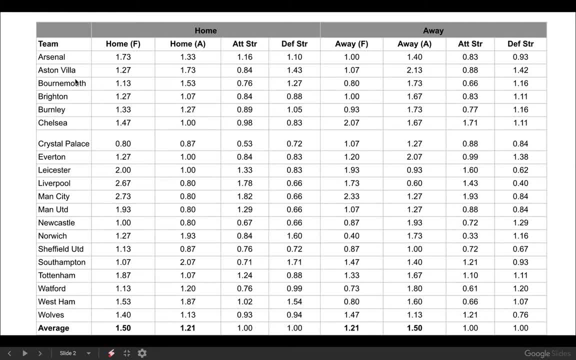 So I haven't excluded the recently promoted teams. I've got all of the teams in the current season, So everything is as you see it. So, firstly, what we need to do is to calculate the average number of home goals scored. 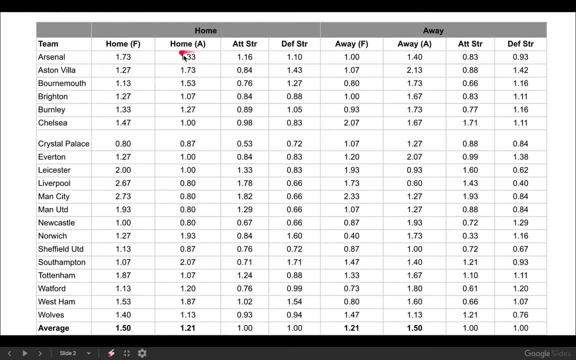 So if we use Arsenal as an example, home goals conceded, away goals scored and away goals conceded. So these are the columns here that we're looking at. So to do that, you just do a normal average calculation. So you go through, find out how many goals Arsenal have scored at home and divide it by the amount of games they've played. 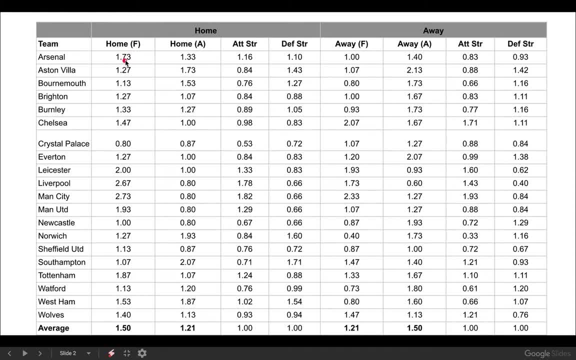 And that comes out at 1.. So 1.73 goals at home on average for Arsenal. We do the same with away goals conceded at home. That A is really it stands for against, but it's really confusing me. So we do the same for the goals conceded at home. 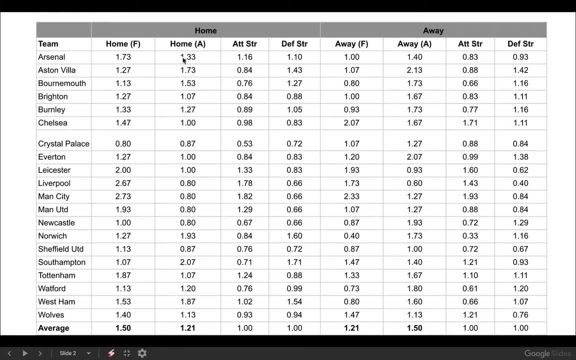 So we're looking at the amount of goals Arsenal have conceded divided by the amount of games they've played, And then we do the same away. So it is Arsenal's away goals scored divided by the amount of games And the goals conceded away from home divided by the amount of games. 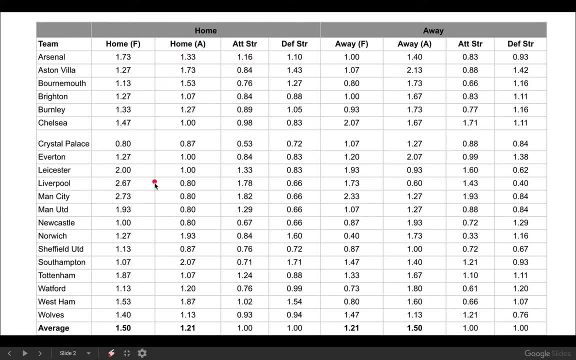 So we do that for all of the teams. That's what we've done here, And that is to allow us to calculate the stat that we actually need for the Poisson distribution model, which is the attacking strength and the defensive strength stats. 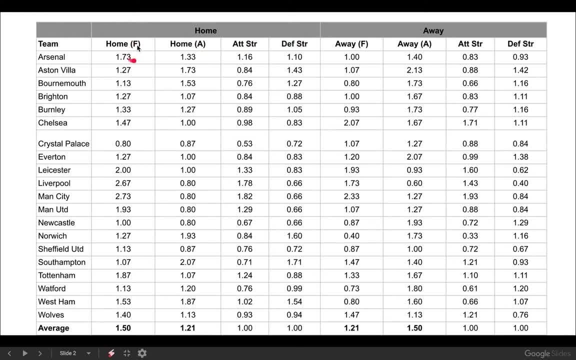 And to calculate these we use the stats that we've got for Arsenal here. For attacking strength at home, we're going to use this 1.73.. And we're going to divide that by the number down here, which is the average. 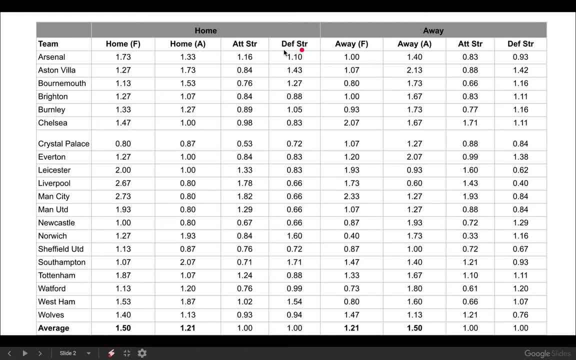 And we come out with 1.16.. And then we're going to do the same for the defensive strength And we're going to use the average, And again for the away we'll do the same. And that's where we get these columns here. 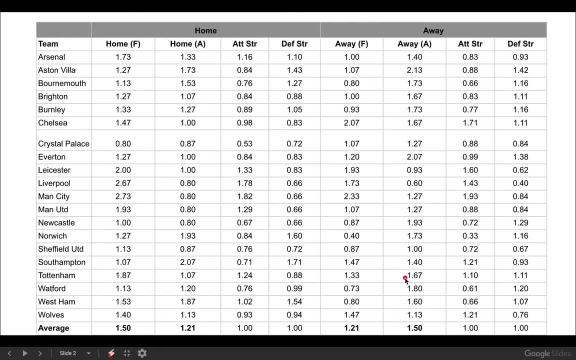 And these are the columns that we're going to need to calculate our Poisson distribution models. The others are not going to be as important going forward. These are the ones we're going to need to calculate the outcomes of games. So, if we skip on to the next slide, I've used Tottenham versus West Ham, which was on the 24th of June 2020.. 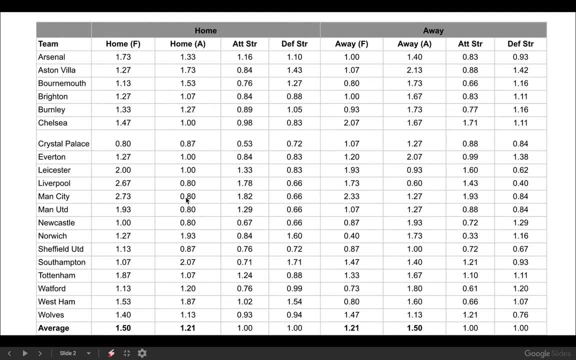 I recorded it before the game was played. actually, I'm quite glad that I haven't had a chance to upload the video until afterwards, just to prove that there was no bias in the result predictions, or I'm only using stats that look favourable. 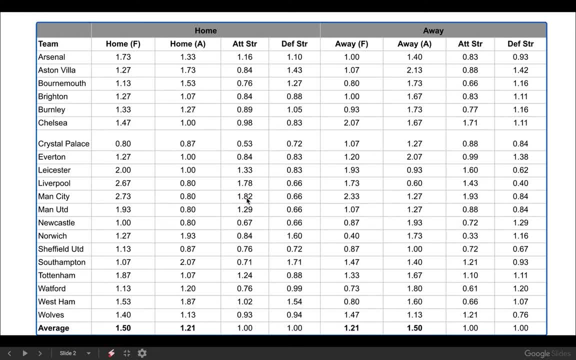 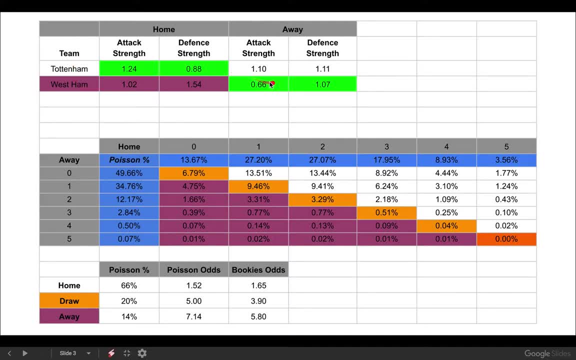 I don't know how favourable they do look, to be honest. So let's have a look So you can see. in slide 2, I've isolated the Tottenham and West Ham stats for you from the previous slide so that it makes it a little bit clearer. 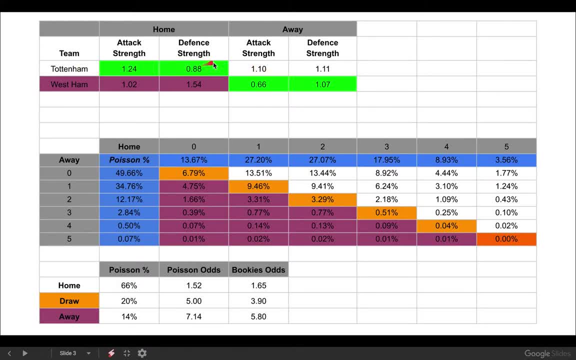 So we've got Tottenham's attacking strength and defensive strength at home. So we've got attacking strength and defensive strength away, and the same for West Ham. Now I've highlighted in green the stats that we're actually going to need to predict the outcome of this game. 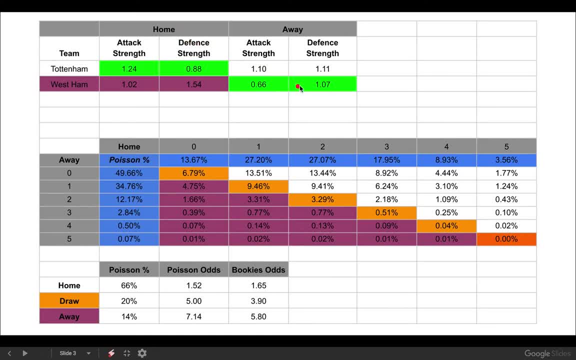 So we're going to need Tottenham's home stats because they're playing at home and West Ham's away stats because they're playing away, And if we look down here, this is the overall result we get coming out of it. 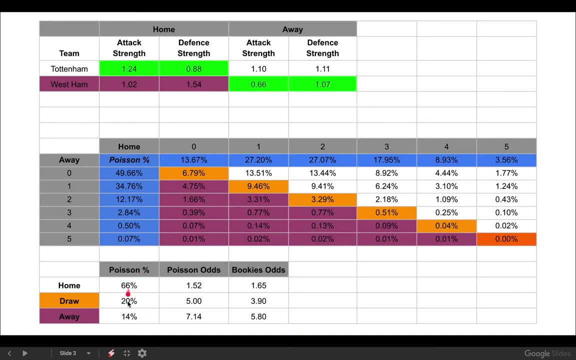 the percentage chance of the outcomes home draw and away. So we've got 66% for Tottenham, 20% a draw and 14% a West Ham win. And the way that we get that is by calculating. 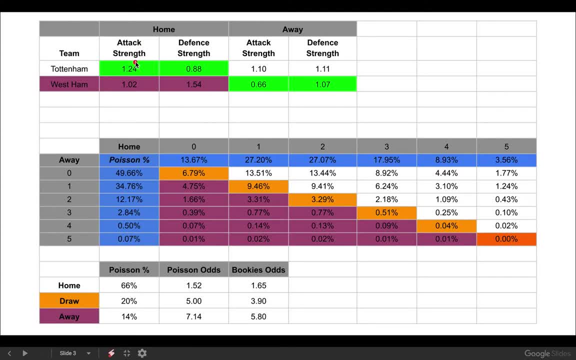 For Tottenham. first we have to find out how many goals they're likely to score, and this is where the Poisson modelling comes in. So you can use an online Poisson distribution calculator to do this, because if you do Google the actual model, you'll see that there's an equation that you can use. 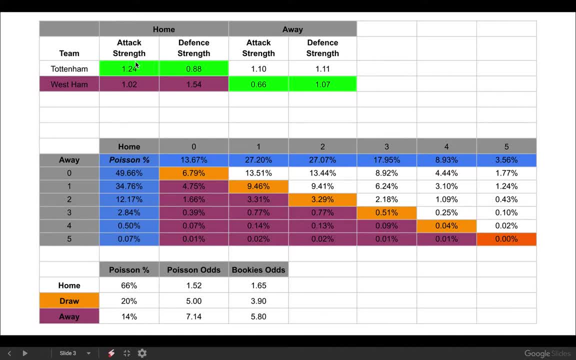 which is pretty confusing, So you can use it and do a walkthrough yourself. but there are Poisson distribution calculators online that are free and easy to use and you punch the numbers in from the attacking and defensive strength and the number of occurrences and you can find out what the percentage is. 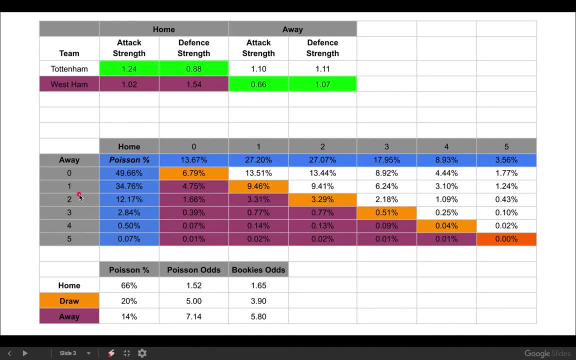 So I've gone from 0 to 5 for home and away, so don't think we're likely to get more than 5 goals per side in the game And the way that these numbers are calculated here. so 1,, 2, 3,, 4, 5,. 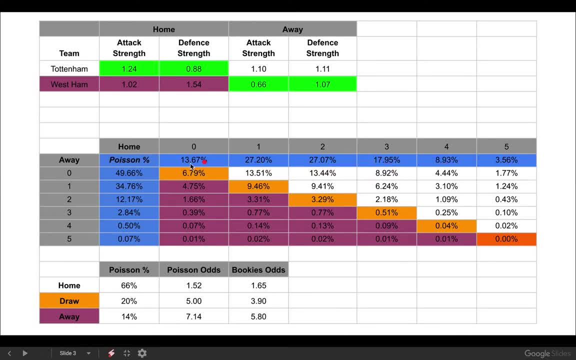 so these are independent of the opposition. This is the amount of times we expect the home team, in this case Tottenham, to score 0 goals, 1 goal, 2 goals, 3 goals, 4 goals or 5 goals. 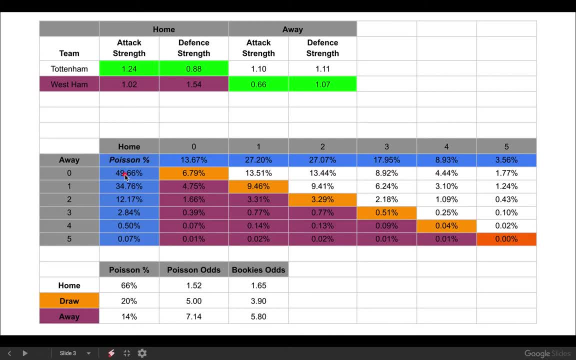 And the same for the away team, in this case West Ham. how often, what percentage of the time, we expect them to score 0,, 1,, 2,, 3,, 4, 5 goals. So this is independent of the opposition. so we're not doing any modelling against the actual fixture here. 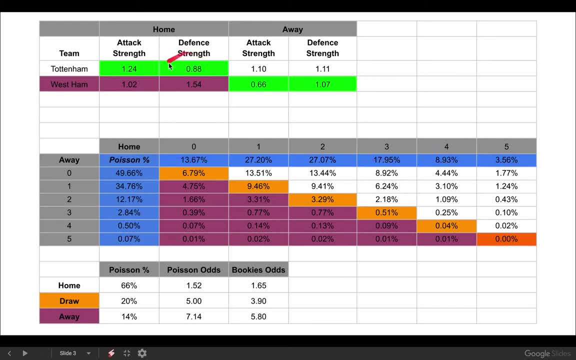 this is just to find out these figures using the attacking and defensive strength, And that's what we've done here. so we can see that we expect Tottenham to score 0 goals just at the 14% of the time. 1 goal just over 27%. same for 2 goals. 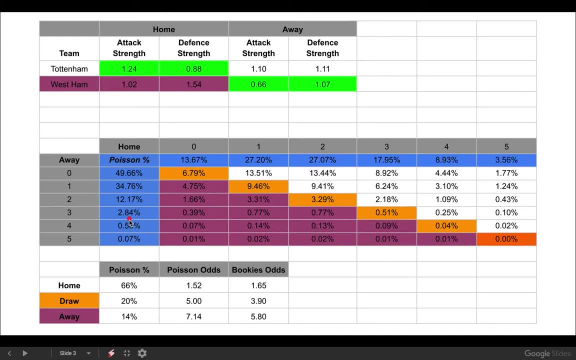 and then 3,, 4,, 5, and the same for West Ham. we've done down here. And then what we do in order to calculate the chances of the actual result, the result of the actual game. so we need to play the 2 stats off against each other. 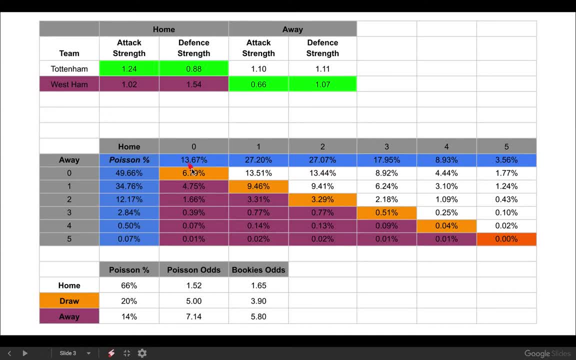 So what we do then is we calculate, we multiply the 2 together and we get the percentage here. So the Poisson distribution model tells us that all of the white ones here these are Tottenham wins, the orange are draws and the colour are West Ham wins. 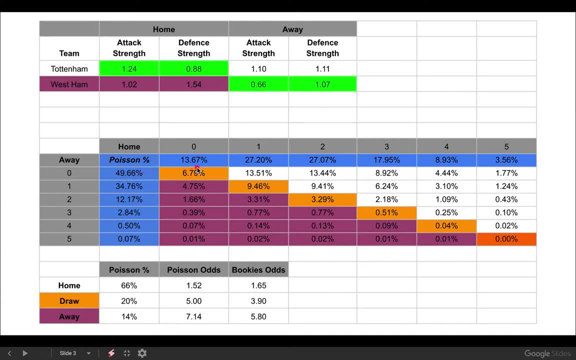 So, looking at this, the most likely result we can see is probably what? 1-0.. So 1-0 looks like just under a 14% chance of a 1-0 win. just under that for a 2-0 win. 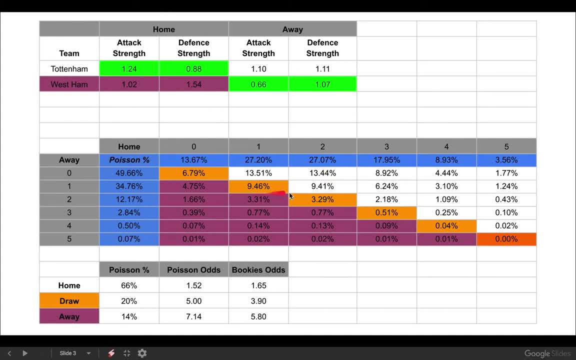 and then you're looking at 2-1,- sorry 1-1, 9.46, and just under that, 2-1 to Tottenham, which is 9.41.. Aside from that, they drop off quite a lot, so we're not really expecting Tottenham to score more than 2 goals. 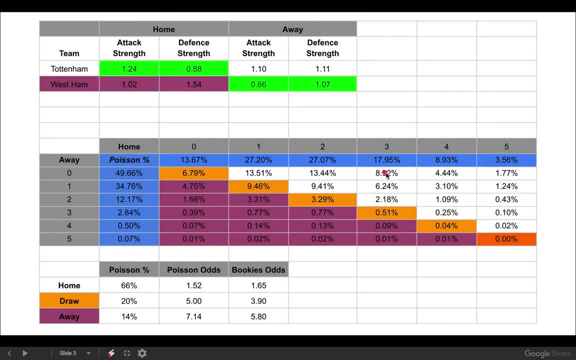 we don't think in this game we've gone from 13.44 to 8.92 here and West Ham. I mean not more than 1 goal at all really. so we're looking at. the result you'd be looking at are 1-0, 2-0, 2-1, 1-1,. 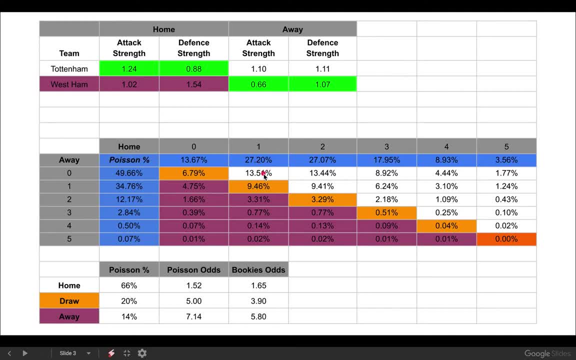 I guess you'd be taking a break. So the highest percentage chance if you were going to purely use this as a model to predict the correct score you'd be looking at, I guess 1-0, very closely followed by 2-0,. 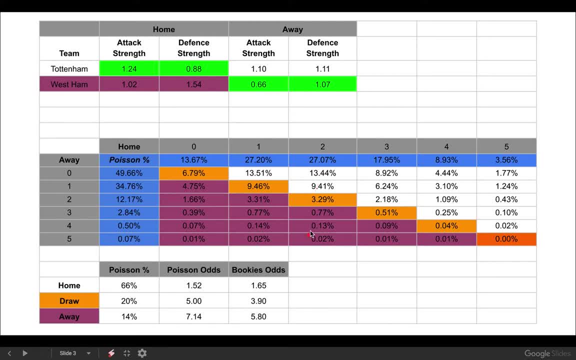 and what we actually saw in the match as it played out. it was 2-0. it ended up, but it was 1-0 until about what? was it the 81st, 82nd minute, and it looked like it was going to be ending 1-0. 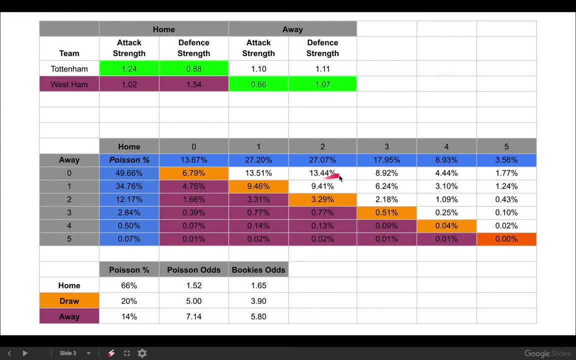 It did actually end in 2-0, because Harry Kane scored fairly late on. I mean, it's not necessarily a fail-proof way of predicting a score, but it's an exact result. I wouldn't usually use it for correct score betting because it's a little bit. 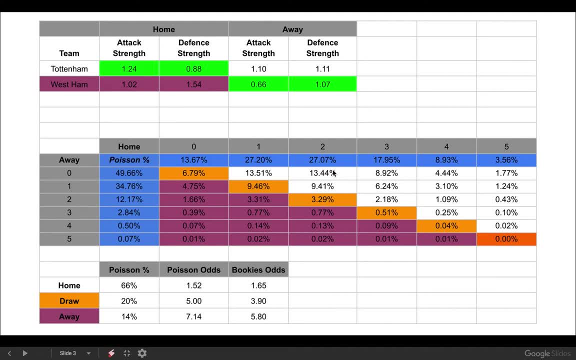 well, as you know, there's so many variables in football that correct score betting is pretty tough. but if you were to use it in this instance, you wouldn't have been far off, and if I ever do do correct score betting, I usually I'll be on the Betfair markets. 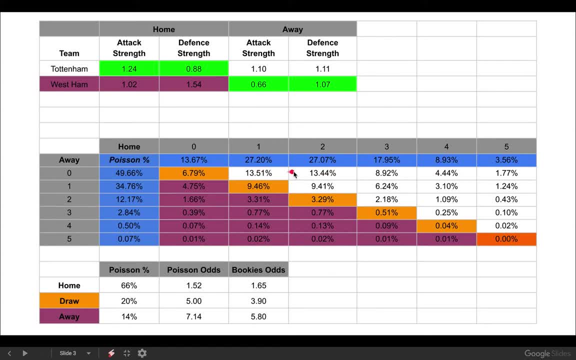 and I'd usually have a couple of different scorelines and I'd trade in and out throughout the match. so I'd definitely have had 1-0, 2-0, and probably 1-1 in this instance and traded as I saw appropriate through the game. 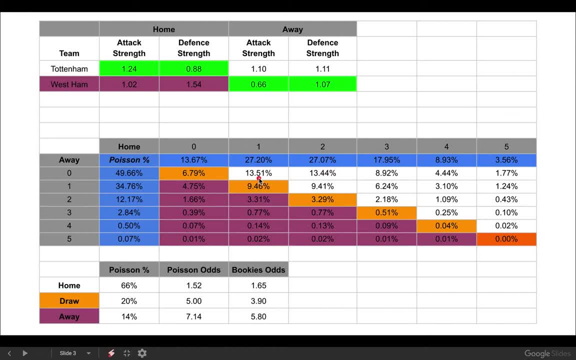 So I think those three results you would be not far off using this model. I tend to use it more as an indicator to tell me what sort of result I should be looking at home away and draw, and how strong that result would be. 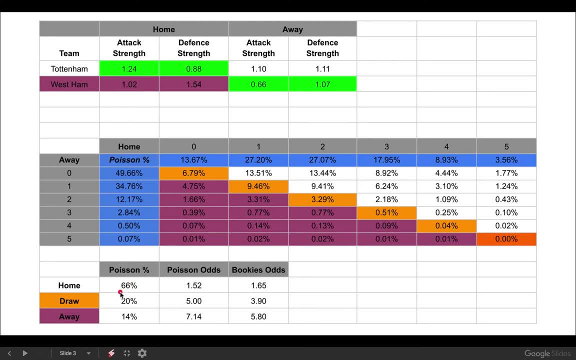 So if we were looking at down here 50% home win, 30% draw and 20% away, maybe I probably wouldn't be lumping on Tottenham because it's going to be a lot closer. I'd probably be going for a draw, whereas 66% you're thinking. 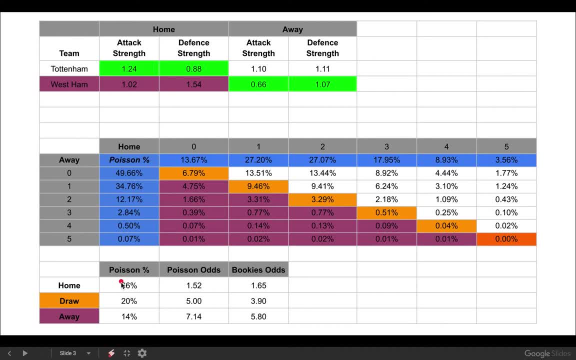 well, the stats do suggest that they're in a good position. and then you've got to put your own knowledge on top of that and you've got to look at team news. you've got to look at your injuries, look at the state of play in terms of the coronavirus, for example. 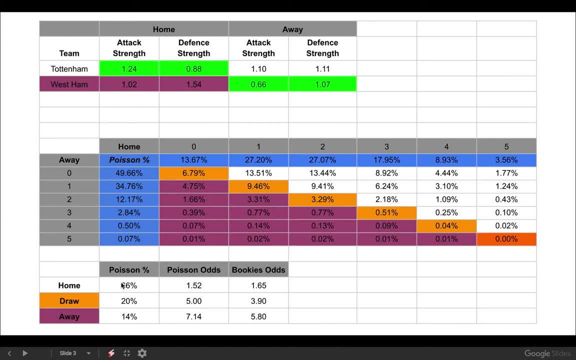 and whether you think that percentage should come down a little bit because we're not looking at the home and away buyers as much. Look at the weather conditions, you know the usual sort of thing. You do need to put that on top. I wouldn't suggest purely going with statistical data. 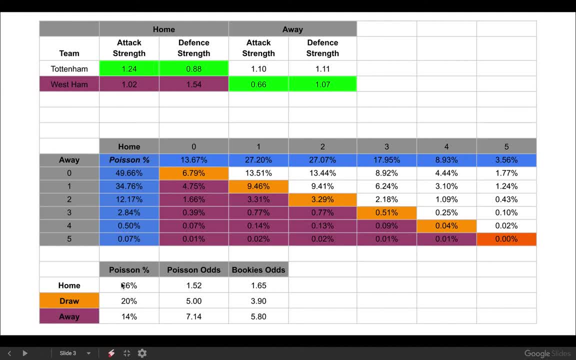 to do football betting because there's so much more to it. But if we do look down here, I've also put in. so this is the percentage we're looking at. Poisson are predicting a 66% chance of a win, 20% draw, 14% away. win. 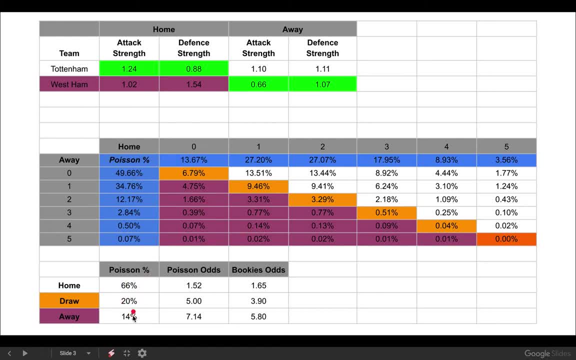 If you add up all of the percentages in these, they might be a couple of percent out, as for example, 60, 80, 90. No, this one does add up, but if you add them up. basically, I've used different rounding rules slightly. 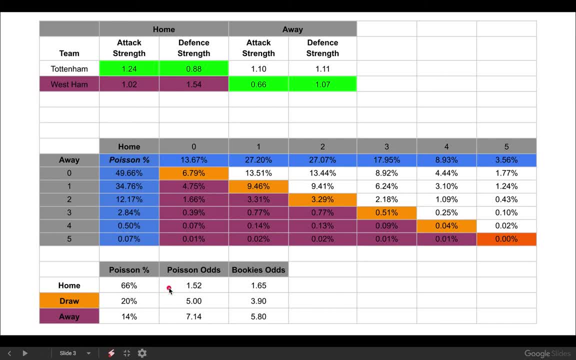 I'm not going to pretend that it's going to be completely accurate, but it is to half a percent accurate, So 66%. and then I've looked a little bit into what I call value betting, and this is something that I'll be doing videos on in the future. 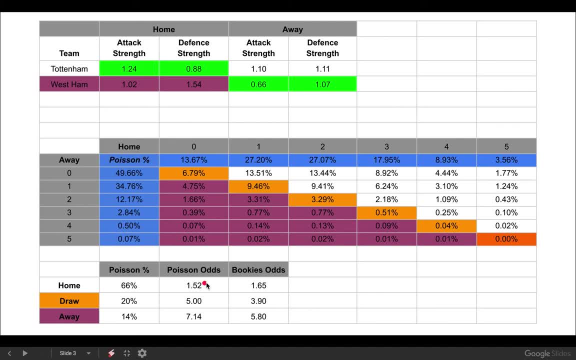 But if you convert 66% of a chance of a home win into odds, then you're looking at about a 1.52 chance in terms of the odds. That's the sort of odds you should be getting- 1.52.. 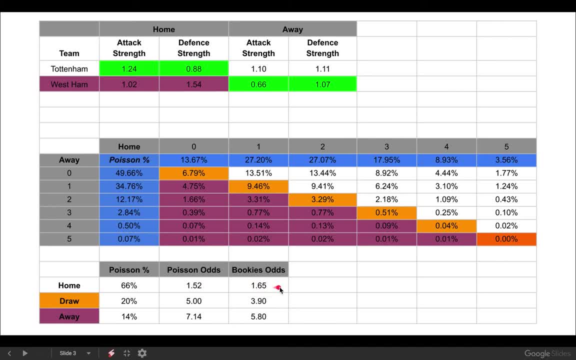 The bookies that I was looking at at the time were actually offering 1.65, so that represents a value bet. So there's value in that. so you could actually put a bet on there. The draw: you should be getting odds of about 5.. You're only getting 3.90,. 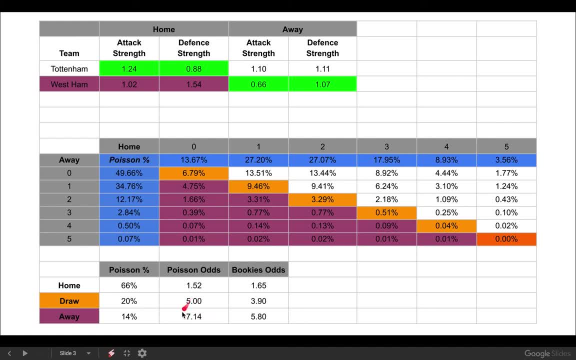 so that's not good value And the away the process. I'm suggesting you should be looking at getting 7.14, and you're only getting 5.80.. So even though it seemed a pretty obvious Tottenham win, the actual value is also still in putting money on a Tottenham win. 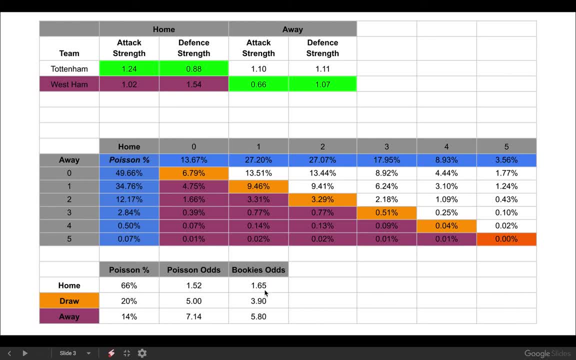 So that might have been able to inform your decision going forward when betting as well. This was a bit of a simple, quick, rough run-through of the portfolio. I hope that you might have found it useful. In the next video, I'm going to be looking at something which I've been working on over the last couple of years. 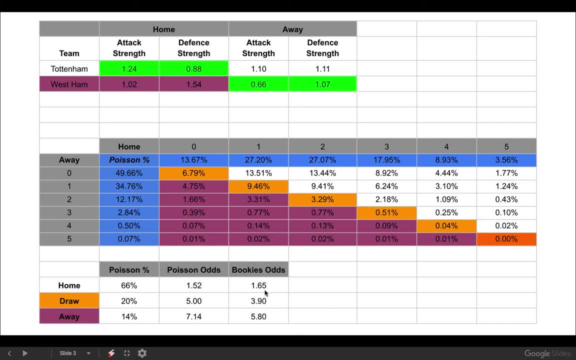 which is quite exciting and that I hope that you might find interesting. and that's my betting strategy that I use to bet on draws. So draw betting is heavily underused in my opinion. Most punters want to see a win, They want to see a goal. 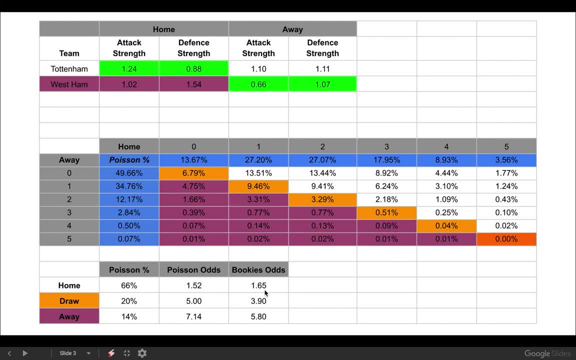 They're not really interested in a dull 0-0 or a cagey 1-1.. And the bookies' odds will normally reflect that, and the amount of money pumped into either the home or the away team winning will mean that the odds for the draw can go up and they're often underutilised.